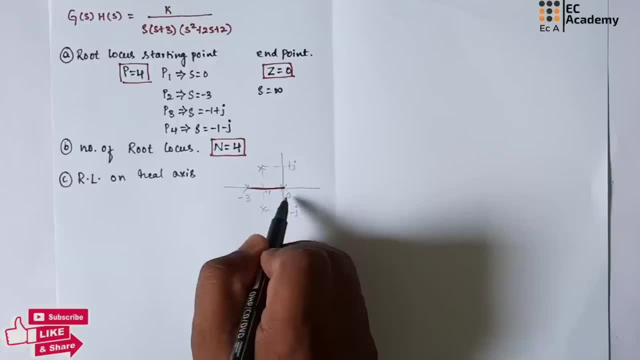 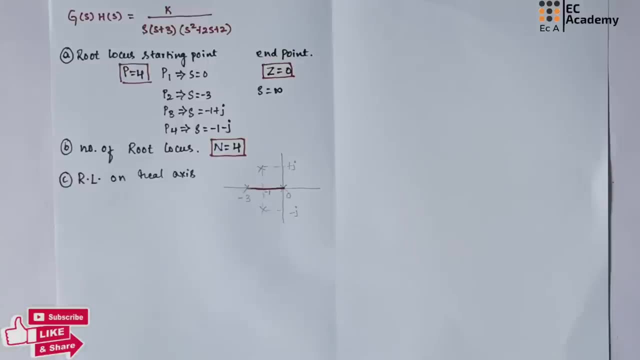 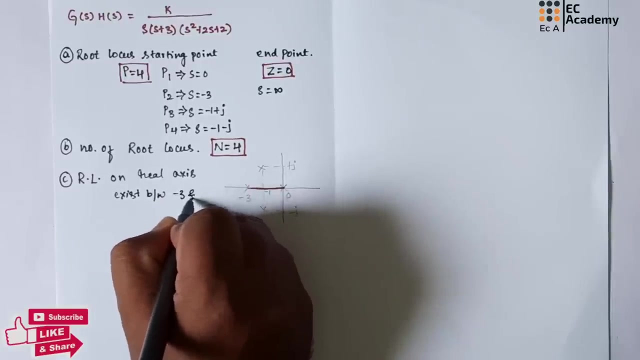 of poles. That's why root locus exists between minus 3 and 0. So 0 is the starting point of root locus. So on the real axis, root locus exists between minus 3 and 0.. Next we need to find number of asymptotes. Number of asymptotes: 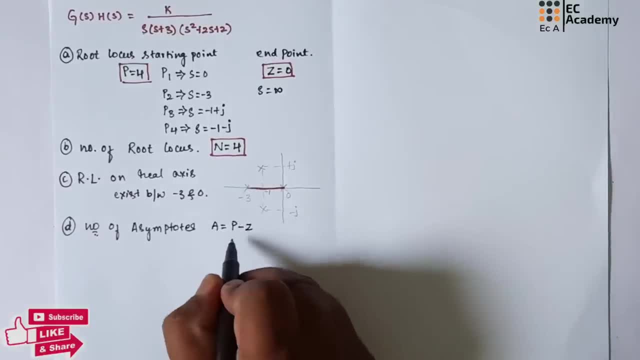 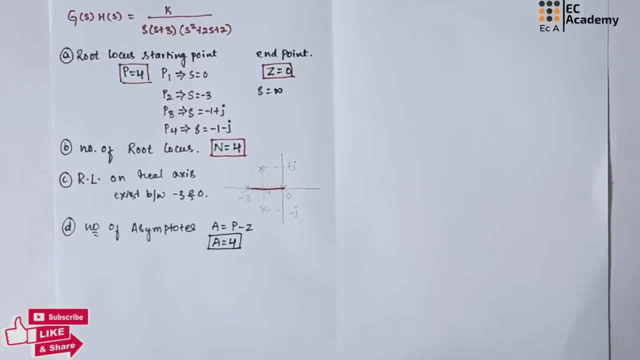 A will be equal to pole minus 0. pole is 4, zeros are 0, so the number of asymptotes is 4. so we will be having 4 asymptotes. now we need to find center of asymptotes. we can write center of asymptotes as sum of poles minus sum of zeros, divided by pole minus zeros. so which means if: 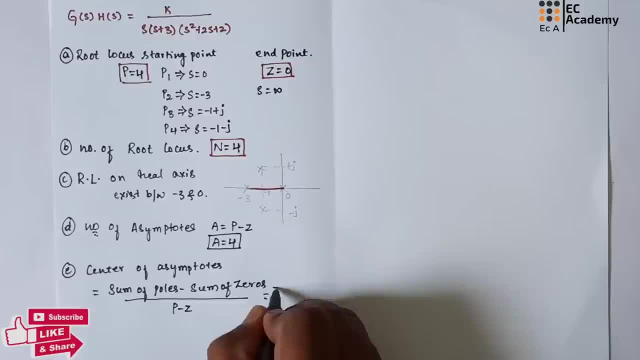 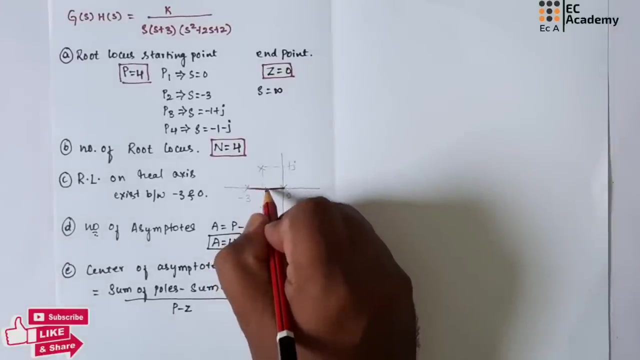 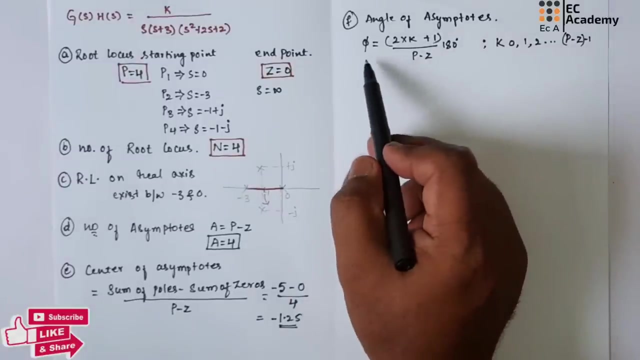 we add all these poles, we will get the value as minus 5, minus 0 divided by pole minus zeros are 4. so we will get center of asymptote at minus 1.25. so somewhere here we will get the center of asymptotes. now let us find the angle of asymptotes that can be given, as 5 is equal to. 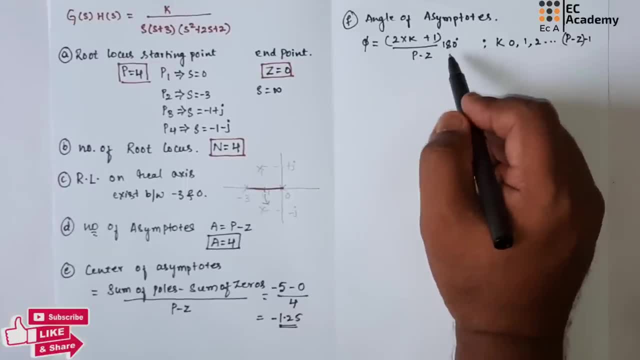 2k plus 1 divided by pole minus 0, so we will get the center of asymptotes at minus 1.25. so somewhere here we will get the center of asymptotes at minus 0 into 180 degree. here k can be given as 0, 1, 2 and so on up to pole minus 0. 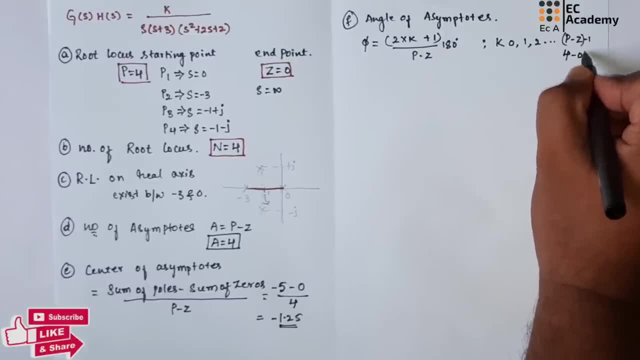 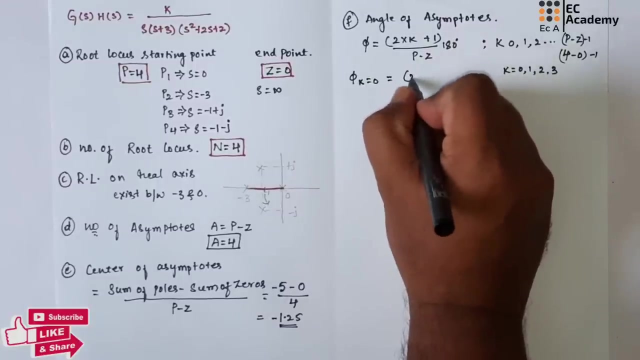 minus 1. so poles are 4 minus 0 minus 1, which means k value will be from 0, 1, 2 and 3. so angle of asymptote for k is equal to 0. can be given as: 2 into 0 plus 1, divided by 4 into 180 degree. 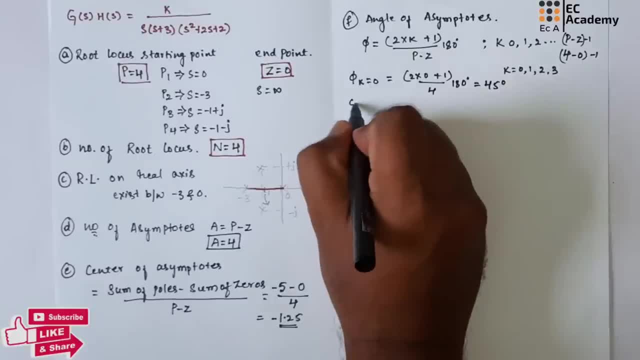 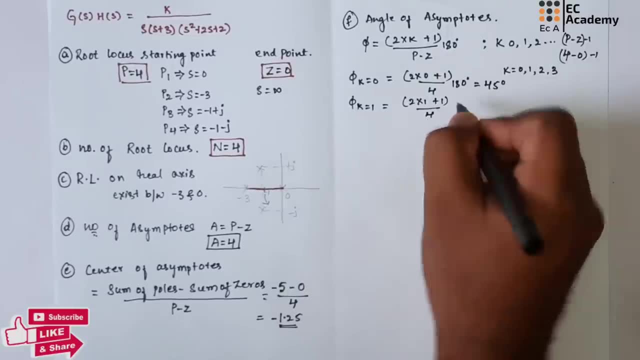 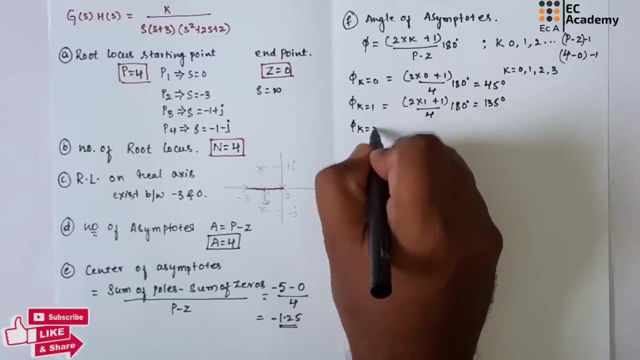 that is nothing but 45 degree. angle of asymptote for k is equal to 1. can be given as 2 into 1 plus 1. divided by 4 into 180 degree, that is nothing but 135 degree. angle of asymptote for k is equal to 2. can be given as 2 into 2 plus 1. 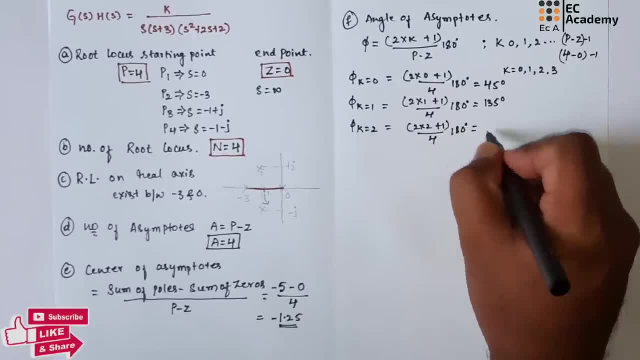 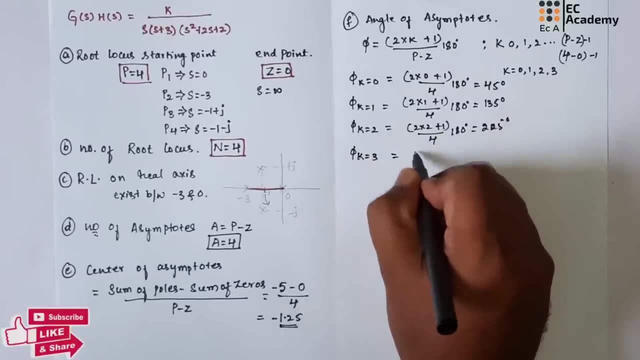 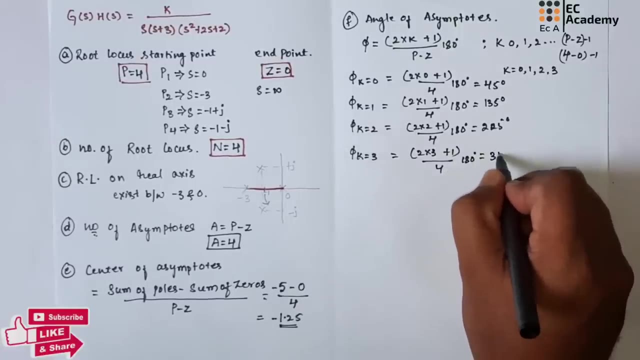 divided by 4 into 180 degree, that can be given as 225 degree. angle of asymptote for k is equal to 3. can be given as 2 into 3 plus 1. divided by 4 into 180 degree, that is nothing but 315 degrees. angle of asymptote as 45 degree. 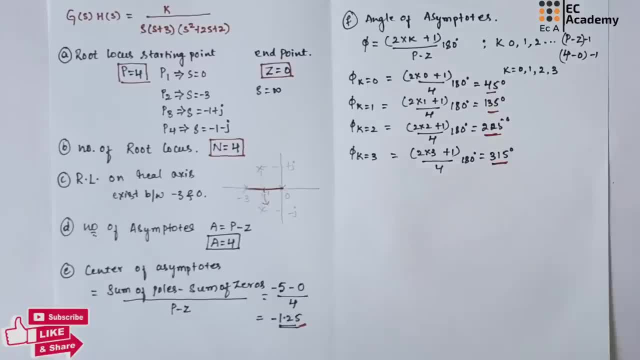 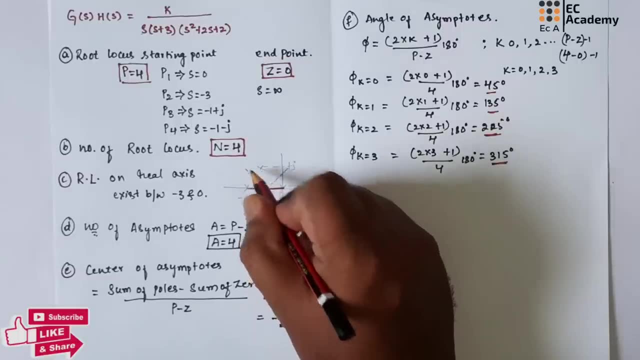 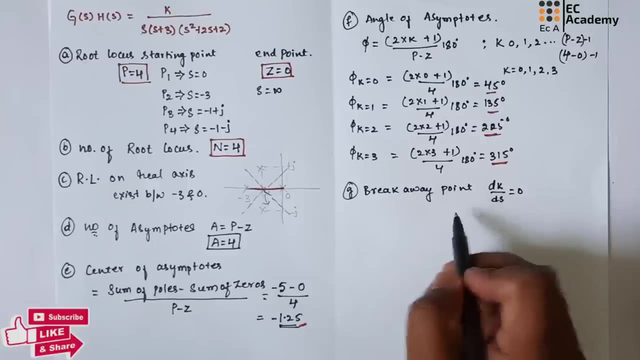 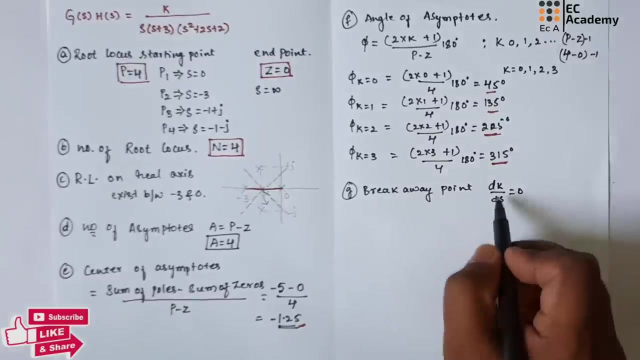 135 degree, 225 degree and 315 degree. so from the center of asymptote we will be having angle of asymptote at 45 degree, 135 degree, 225 degree and 315 degree. Next, let us find breakaway point. We can find breakaway point by taking dk by ds and equating that to 0. So here: 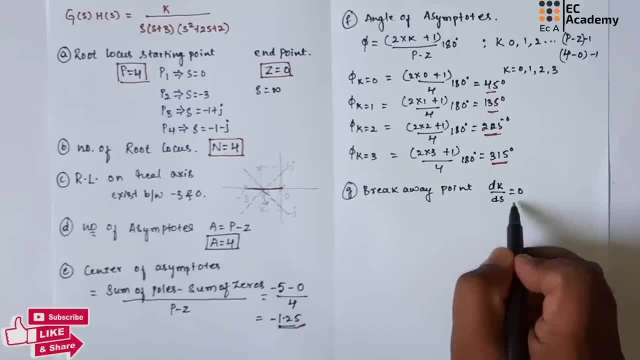 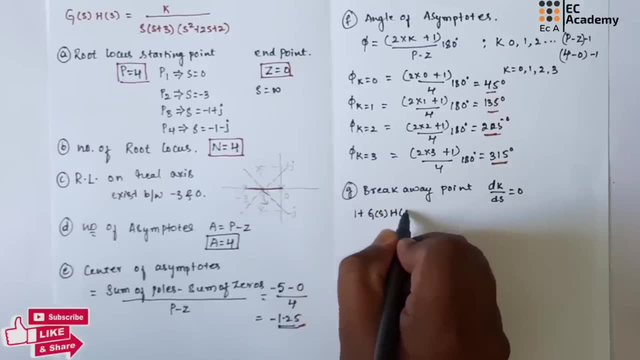 the k value is differentiated with respect to s and it is equated to 0. to find the breakaway point Now, let us consider: 1 plus g of s into h of s is equal to 0. At that case we can take the same. 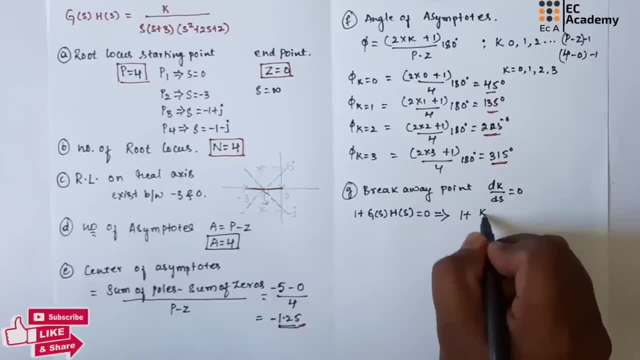 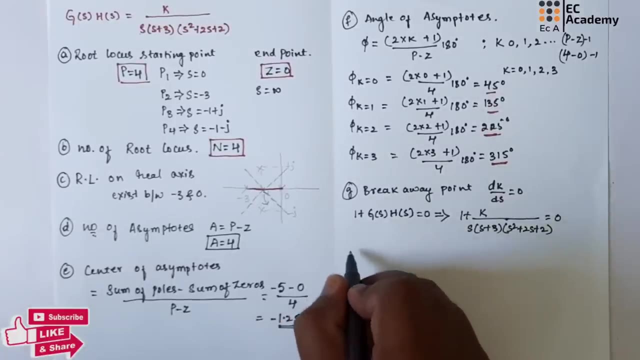 transfer function and we can write 1 plus k, divided by s into s plus 3 into s square plus 2s plus 2 is equal to 0.. From this expression, if we take LCM, we can find the characteristics equation as: s to the power of 4 plus 5.. 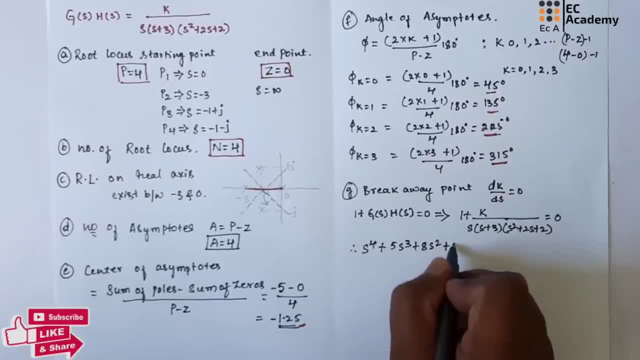 5s cube plus 8s square plus 6s plus k is equal to 0.. So from this we can say k is equal to minus s, to the power of 4 minus 5s cube minus 8s square minus 6s. Let us call this: 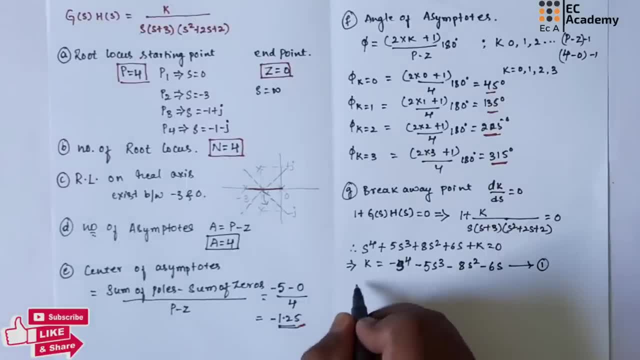 as equation number 1.. For this value of k, let us differentiate with respect to s. So if we differentiate with respect to s, we can say k is equal to minus s, to the power of 4 minus 5s, cube minus 6s, square plus 6s plus 6s plus 6s. So if we differentiate this, we will get minus. 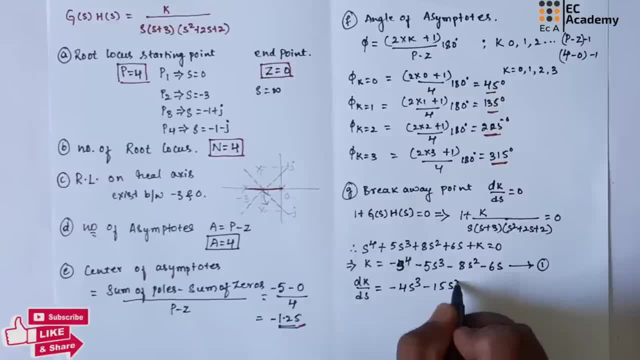 4s cube minus 15s square minus 16s minus 6 is equal to 0.. So this differentiated equation will equate it to 0.. So all the negative terms we can write as positive terms. So 4s cube. 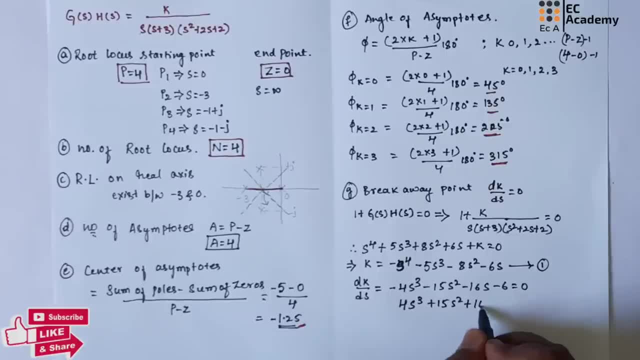 plus 15s square plus 16s plus 6 is equal to 0.. If you find the roots of this equation, we will get three roots. First root is: s is equal to minus 2.288, and we will get two complex root. 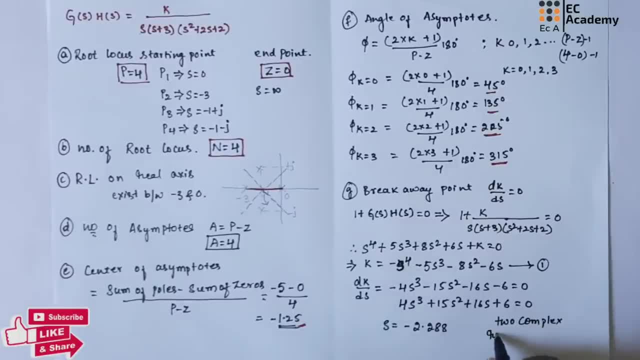 with real part minus 0.7307.. So this complex root will not be available on the root locus. So s is equal to minus 2.288 is the actual breakaway point. So at 2.288 so we will be having the 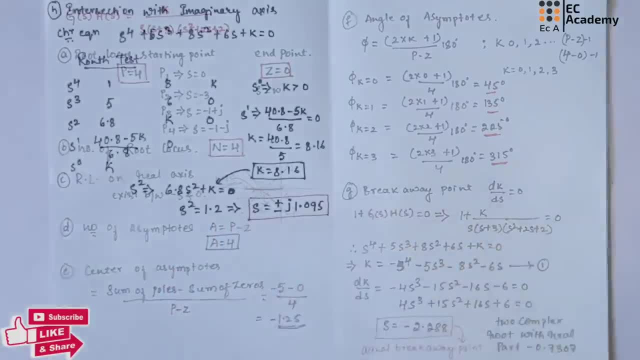 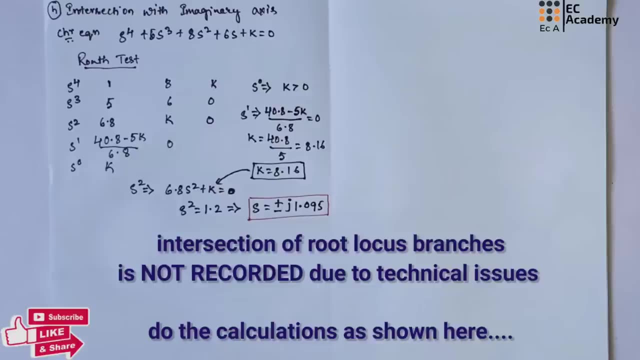 breakaway point. Next, let us find the intersection of root locus branches with imaginary axis. To find this, we will consider the characteristics equation and we will perform rod test on this characteristics equation. From row s to the power of 1, we can find the value of k, which is equal to 8.16.. From row s square, we can write the: 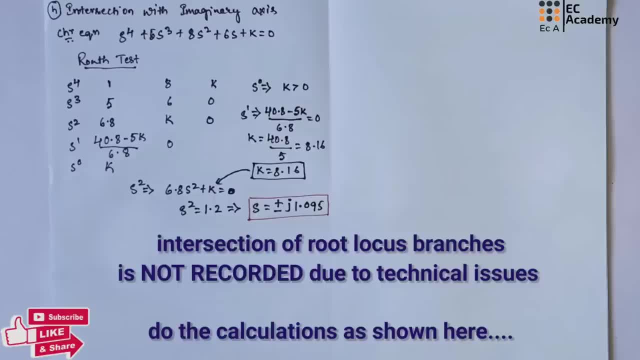 axillary equation: 6.8 s square plus k is equal to 0.. In this, let us substitute the value of k. we can find the value of s, which is intersection of root locus branches with imaginary axis. So the value of s will give us the intersection of root locus branches with imaginary axis. 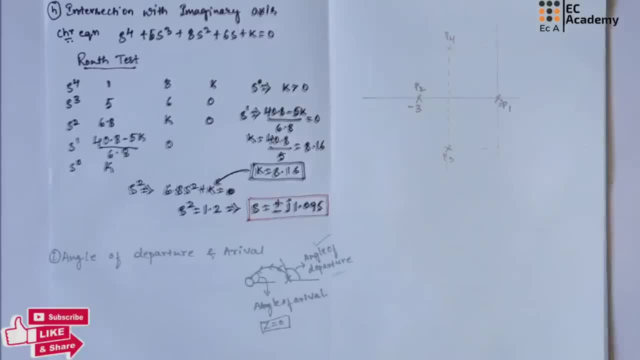 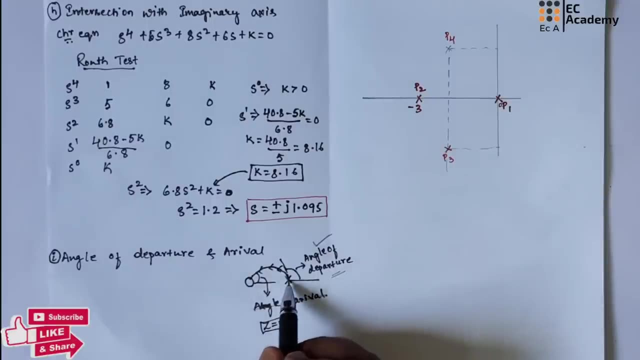 Now let us find angle of arrival and angle of departure. Always remember, when there is a pole and zeros in a root locus, always pole will move towards 0 and the angle at which the pole move towards 0 is known as angle of departure and the angle at which pole arrive at zeros are known as. 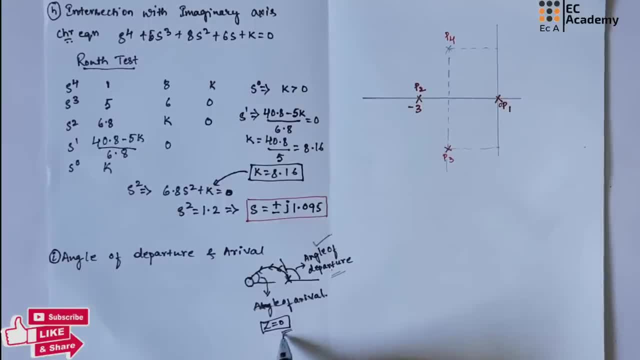 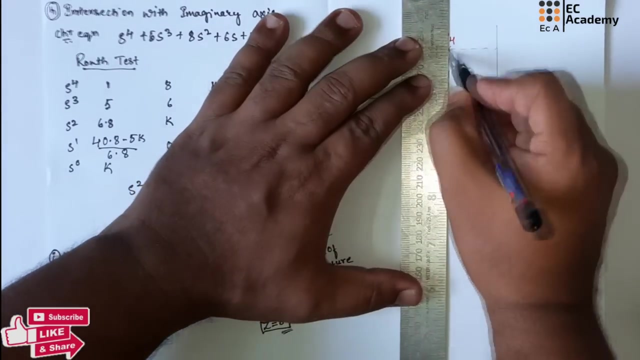 angle of arrival. In this example, we don't have any zeros. That's why we need not find angle of arrival only, we need to find angle of departure. in this problem Now, we need to consider all the poles and we need to join all the poles. So let us join all the poles. 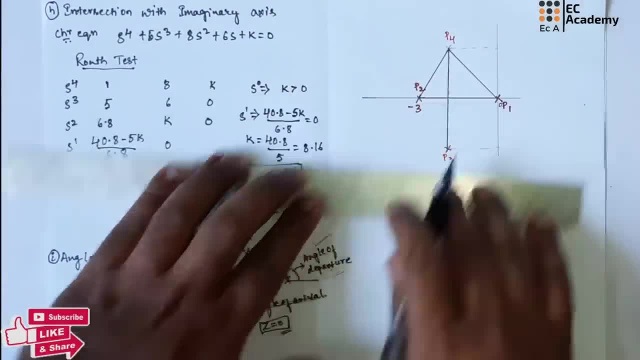 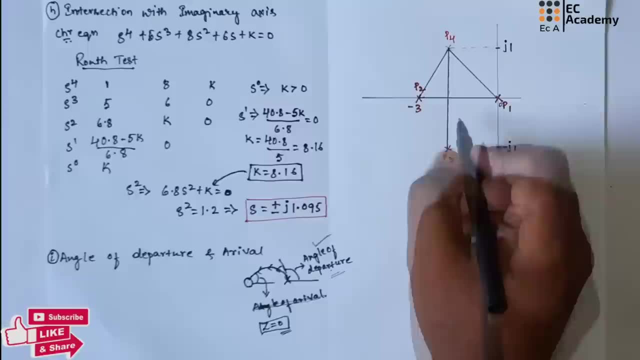 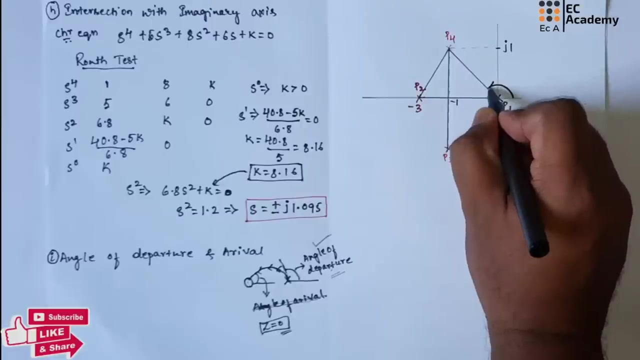 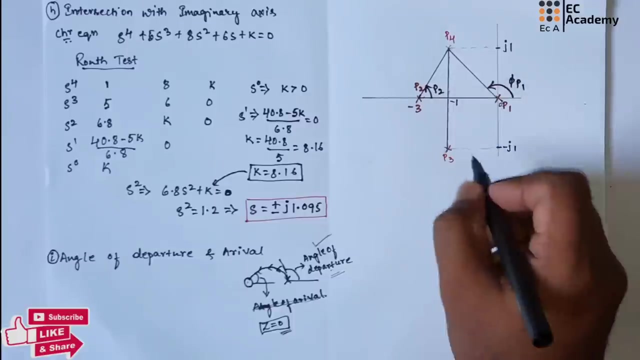 So this is j1, this is minus j1, this is minus 1.. Now we need to find angle at pole 1.. Now we need to find angle at pole 2.. We need to find angle at pol3.. Now let us start again. the right side. We have now taken angle of arrival 0.6 in the left side. This is Powder, one by Pol 3.. So now, oops, I have taken angle of arrival 0.6 in thisisp. дан kennt lang. The angle of the problem now was with minus 0.6 Potatoes, beautiful idea. So this is J1. we have to find angle of departure in this problem and the angle at which pole arrive at zero. 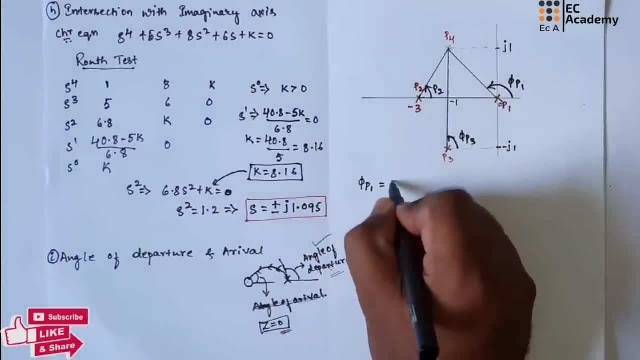 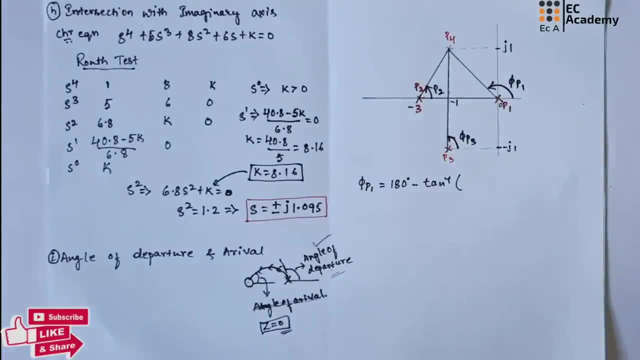 let us find the angle at pole, one that can be given as 180 degree minus tan, inverse of. so first we need to consider this value from this point to this point. so the value is one, so we'll consider then this value. so from zero to this point, we are having the value as: 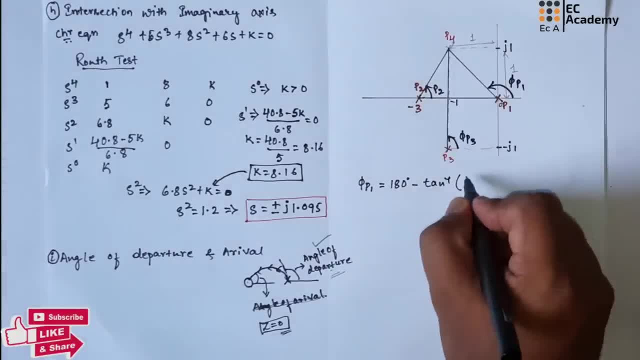 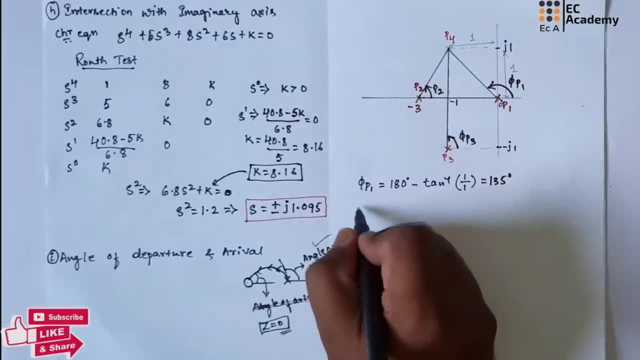 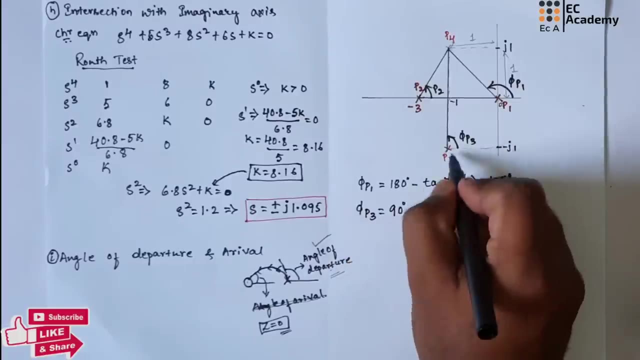 one. so that's why we'll take tan inverse of one divided by one, tan inverse of one divided by one, so this is 135 degree. then we'll find the angle at pole 3. so angle at pole 3 it is 90 degree. so from this point the angle is 90 degree. then let us find the angle at pole 2, so the angle at pole 2. 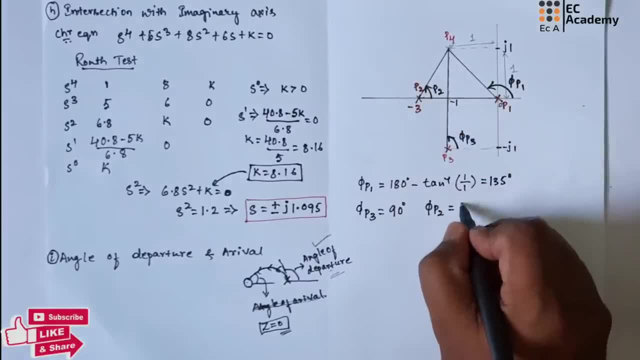 is equal to angle at pole 2, we can write it as tan inverse of. so this value, from this point to this point, it is 1, and from minus 1 to this point minus 3, the value is 2. so it will be tan inverse of 1 by 2. so this is nothing but. 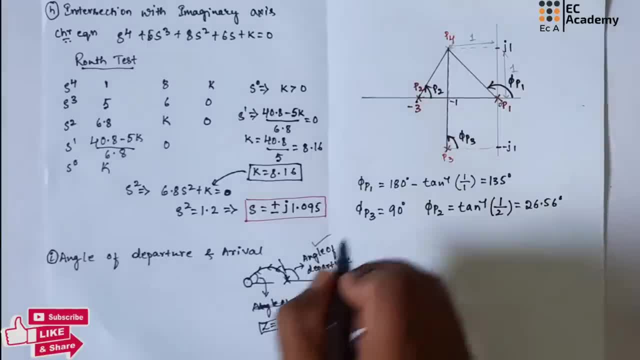 26.56 degrees. now we need to find summation of angle of poles. so we need to add all this angle of poles. so if we add 135 degree, 90 degree and 26 degree, we'll get 251.56 degree. summation of angle of zeros. 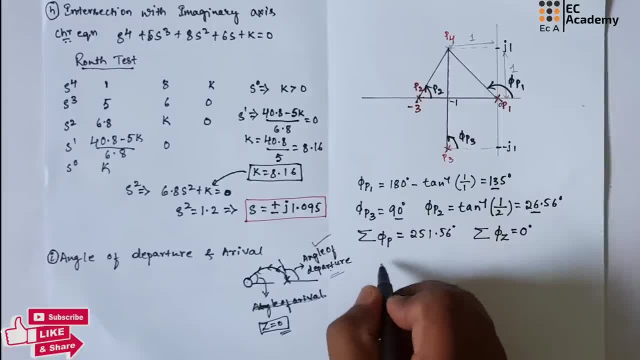 we don't have any zeros. that's why it will be zero degree. so the angle of departure will be equal to 180 degree minus phi. so here phi will be equal to summation of angle of poles minus summation of angle of zeros, so phi value will be equal to 251.56 degrees. so here the angle of 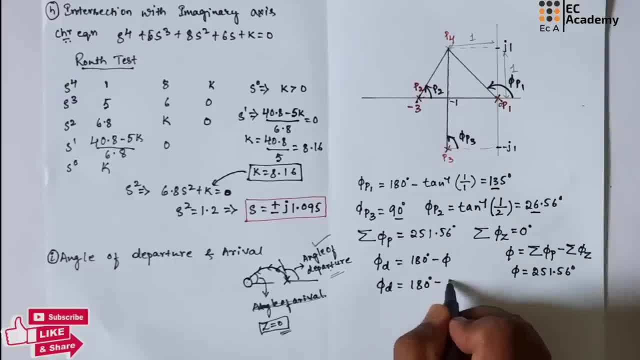 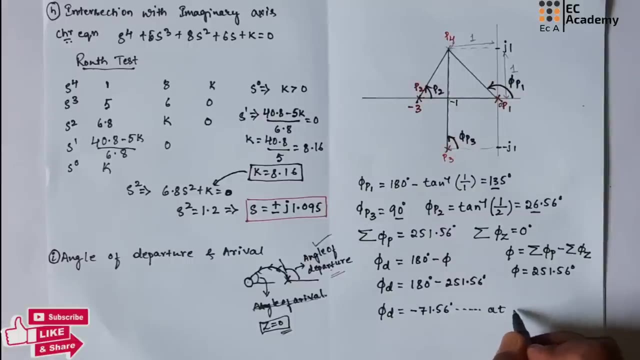 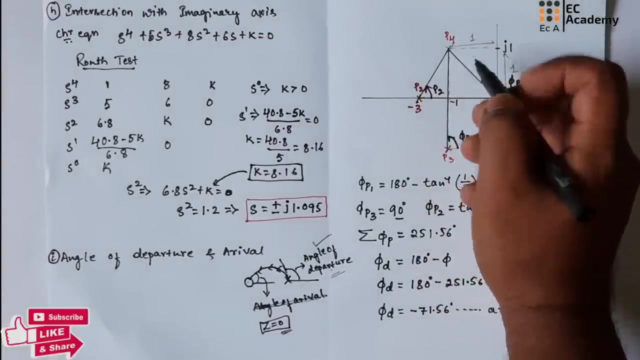 departure. we can write it as 180 degree minus 251.56 degrees, so angle of departure will be minus 71.56 degree. so this will be at minus 1 plus j. so at this point it will be minus 71.56 degrees and angle of departure 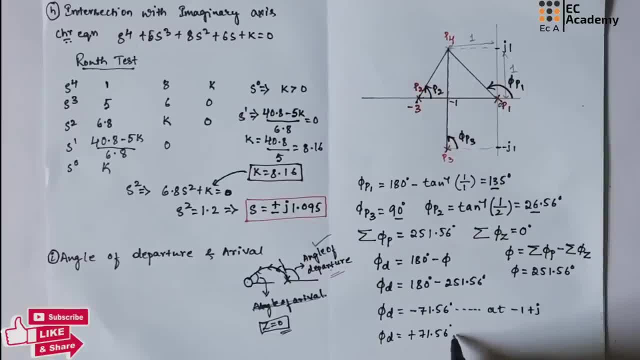 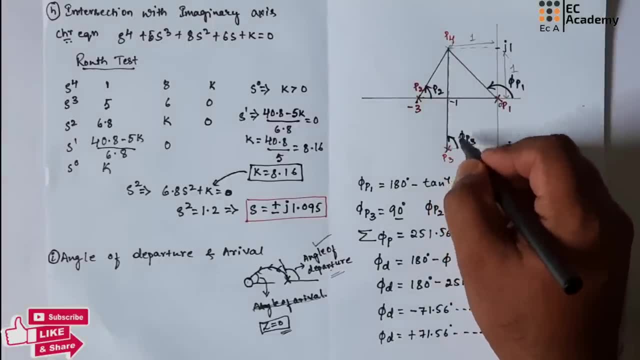 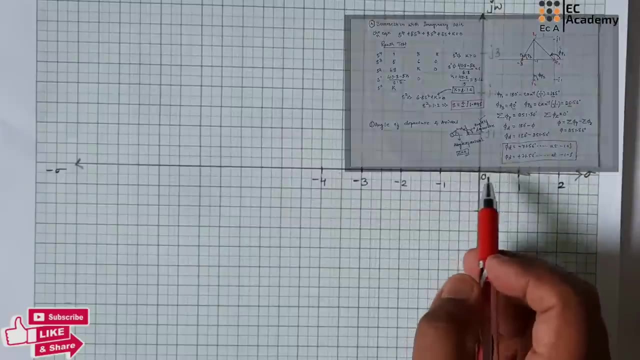 will be equal to plus 71.56 degrees at minus 1 minus j. so at this point the angle of departure will be plus 71.56. now let us plot these things in graph sheet. now let us consider an s plane. in this s plane, let us first mark the. 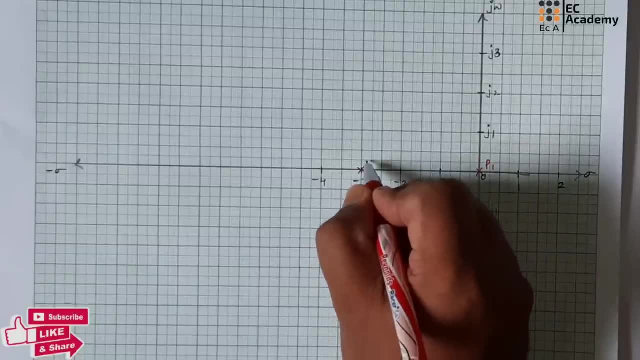 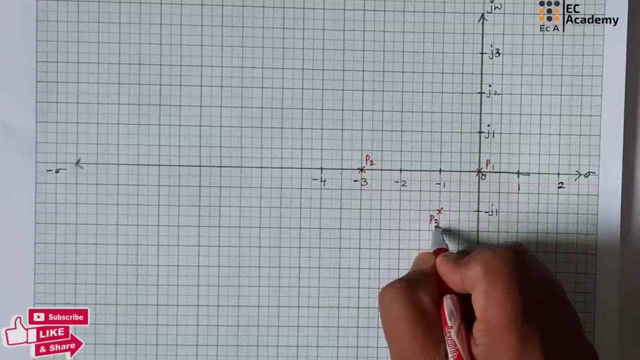 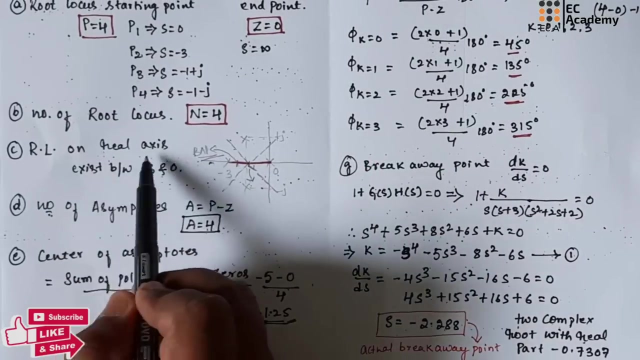 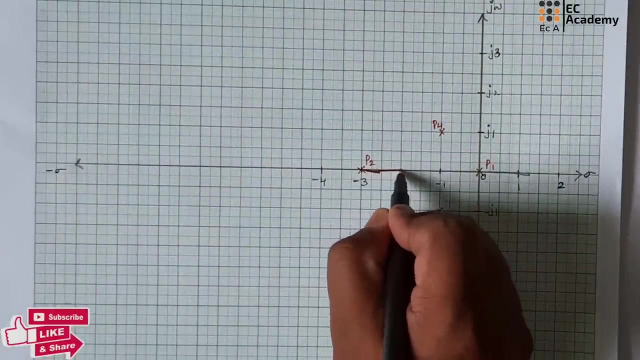 poles. this is pole one at zero. this is pole 2 at minus 3, pole 3 at minus 1 minus j and pole 4 at minus 1 plus j. now the root locus on real axis exit between minus 3 and 0. so the root locus will be between minus 3 and zero. okay, this is the root locus. now there are four solubilities, which are pleasant, because if i rewrite the value of 3 on the threshold as 0.3 and create a single constant, atmediate it soil Prop dan x, 0. study and remember thatạn断 tang and pole 4 are equal to zero and pole 2 is 0 and 0.3 are equal to 0 and ∼1. 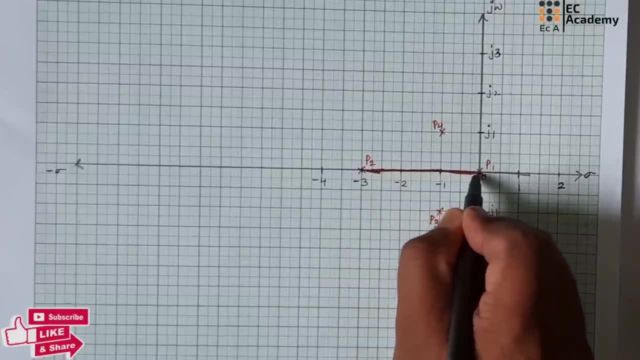 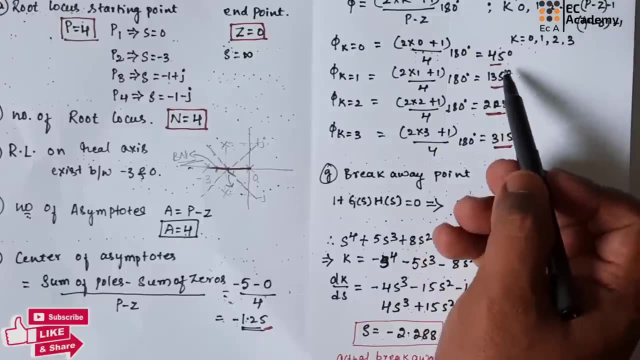 so, on the Pro noch Negowei's analysis, we found that 3 and 0,. okay, this is the root locus. Now there are four asymptotes. center of asymptote is at minus 1.25 and each asymptote is at angle of 45 degree, 135 degree, 225 degree and 315 degree. 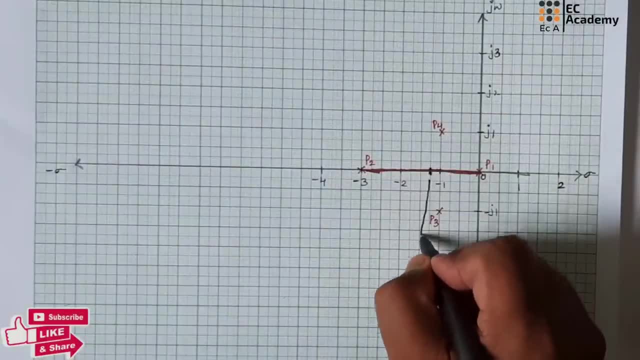 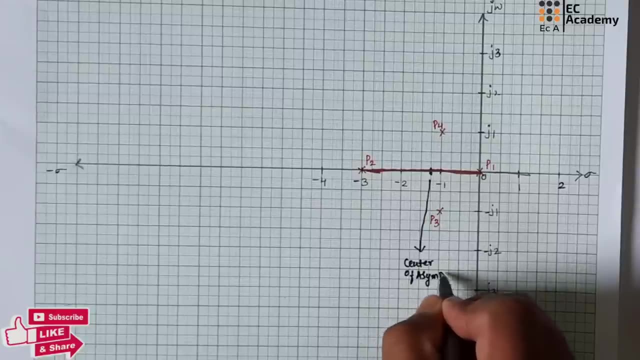 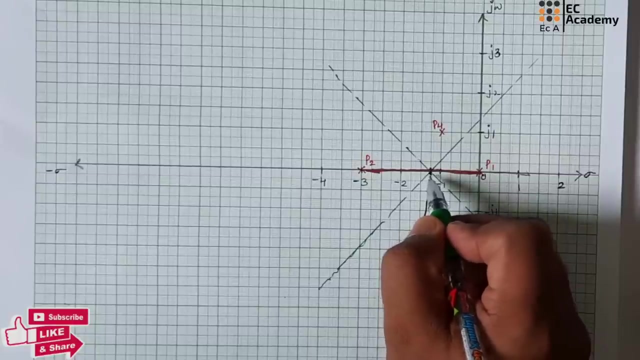 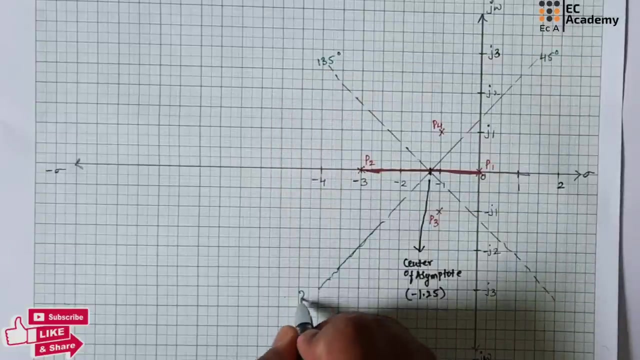 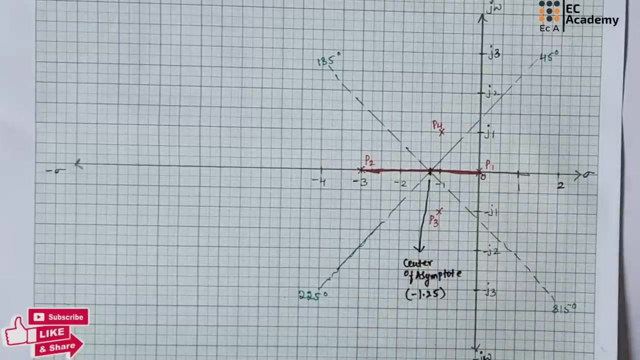 So this is the center of asymptote, So which is at minus 1.25.. From this center of asymptote there are four angle of asymptotes: at 45 degree, 135 degree, 225 degree and 315 degree. So these four are the angle of asymptotes. 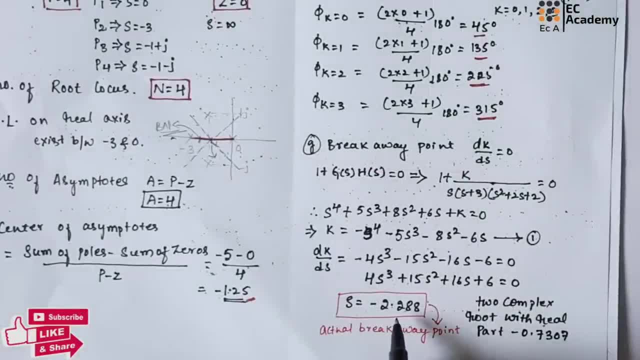 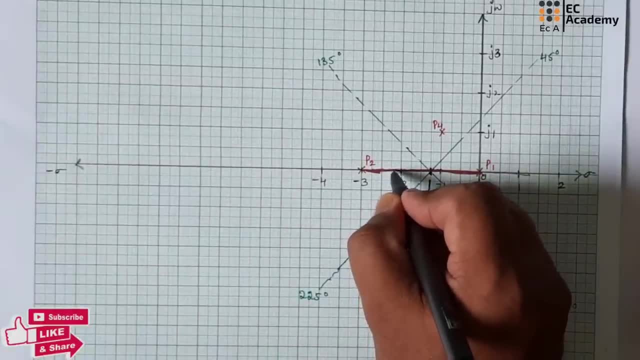 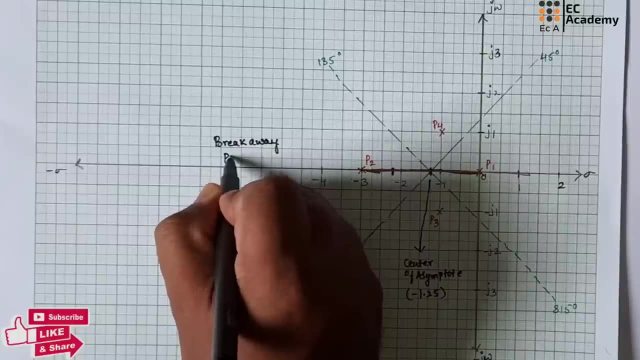 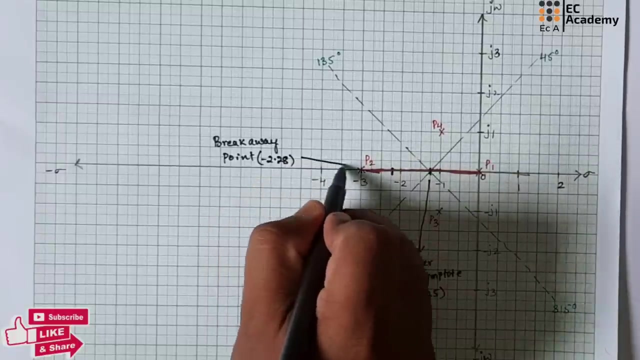 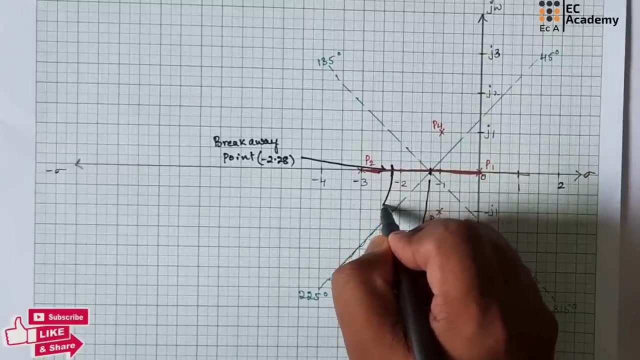 Next, the breakaway point is at minus 2.288.. So the breakaway point is at minus 2.288.. So this is breakaway point at minus 2.288.. So this is breakaway point. So from this breakaway point, root locus branches will move to infinity. parallel to this asymptotes: 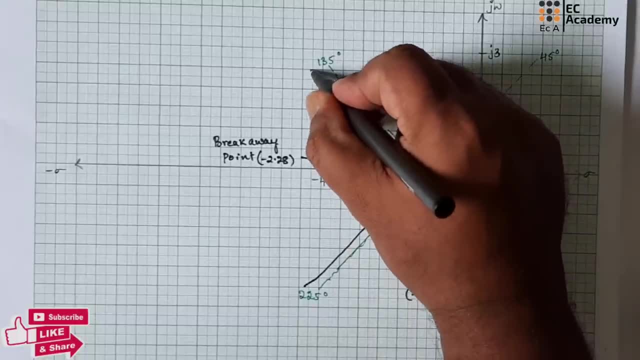 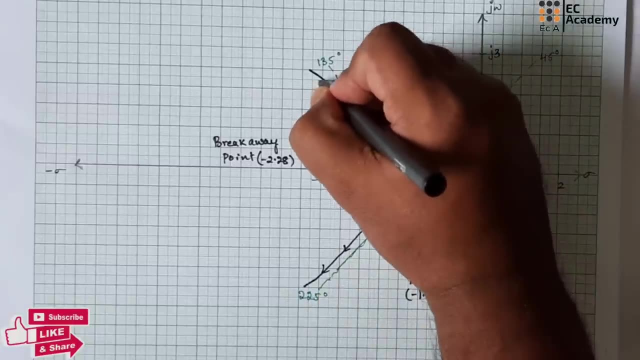 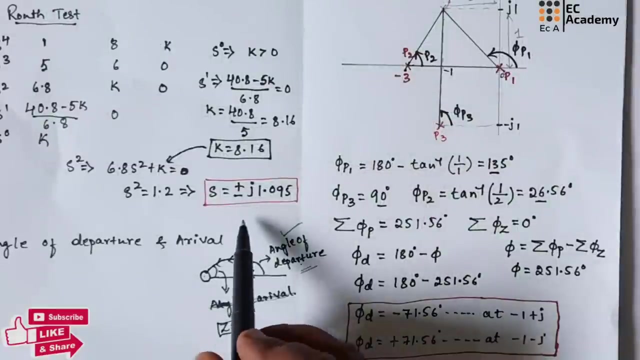 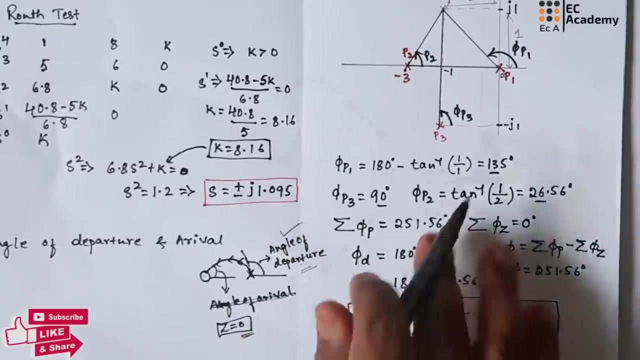 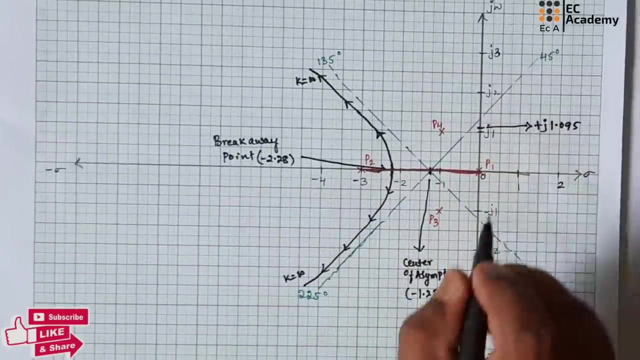 So they will move towards infinity parallel to this. So this will move up to infinity. k is equal to minus infinity. Next, the intersection of root locus branches will be at plus or minus j 1.095.. So this will be the point, plus j 1.095, and somewhere around here it will be: 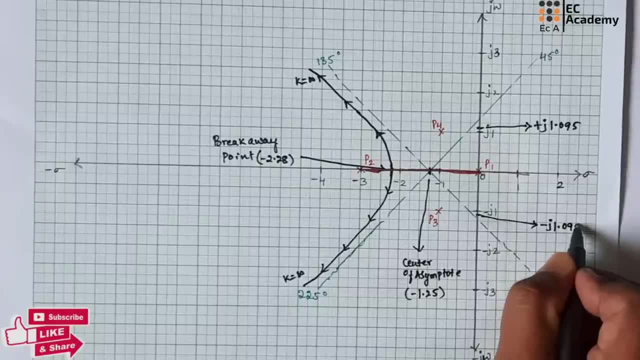 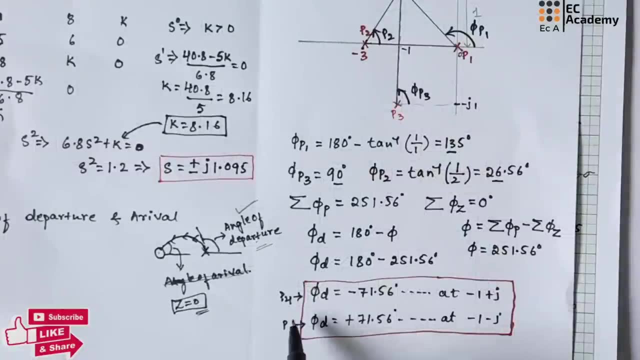 So this will be the point plus j 1.095.. So these two are the breakaway point of root locus with imaginary axis. The angle of departure at pole 4 is at minus 71.56 degrees And the angle of departure at pole 3 is at 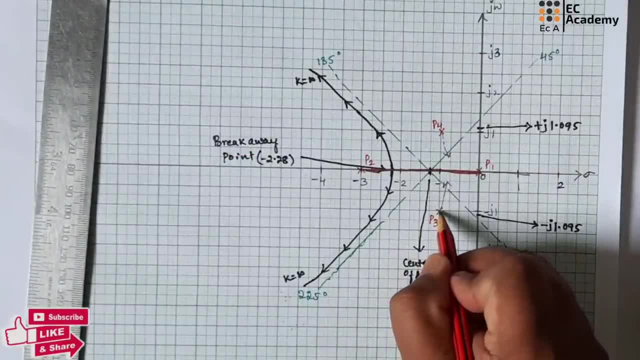 plus 71.56 degrees. So at pole 3 it is plus 71.56 job. So at pole 3 it is plus 74.56 degree And at pole 3 it is at plus 75.12 degree. It will go to 0.276.. And at pole 4 it will come to 0.126 degrees And at pole 5 it will come to1.174.. In other word, this 0.. 작업 we area of AR2.. Also, you will need to learn functions. 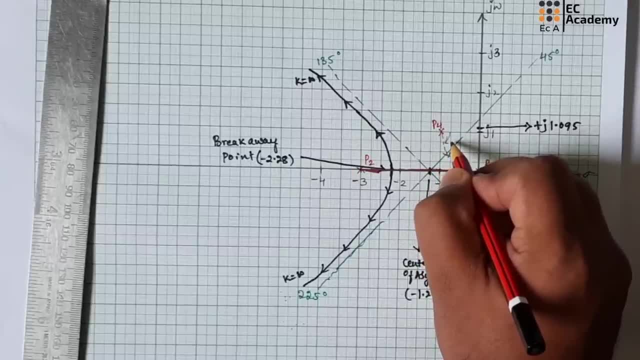 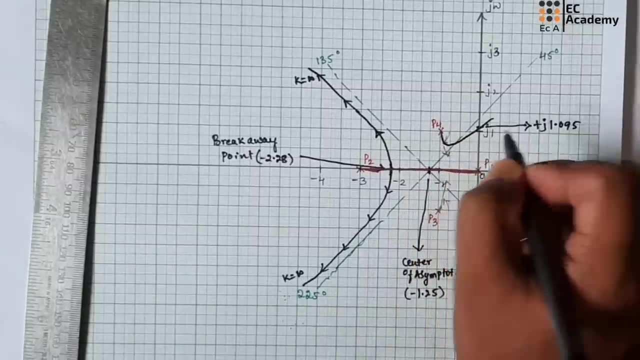 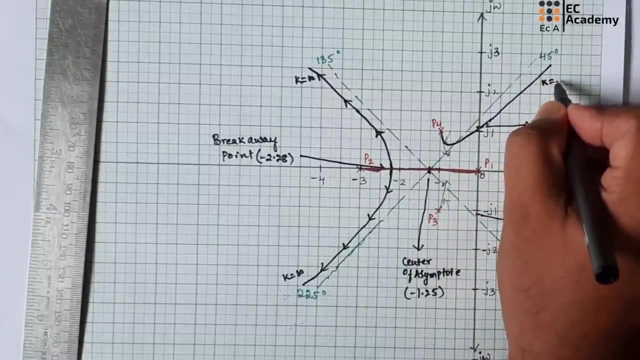 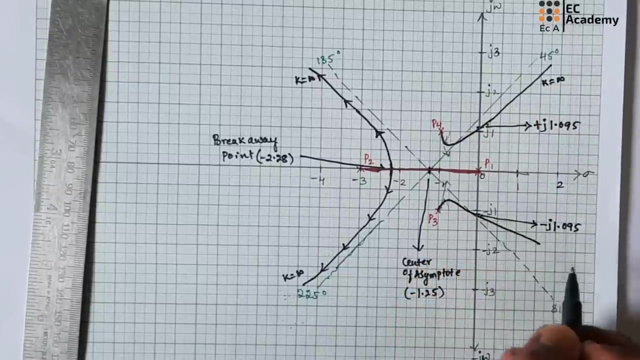 Because all things will be given by the 마음 armored to monitoronneàng. for it is minus 71.56 degrees. so from this pole it will move, intersecting this imaginary axis. it will move up to infinity. K will be equal to infinity in the same way, so it will move, intersecting this imaginary axis, parallel. 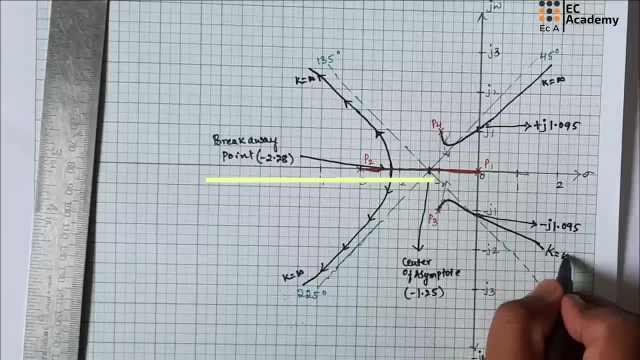 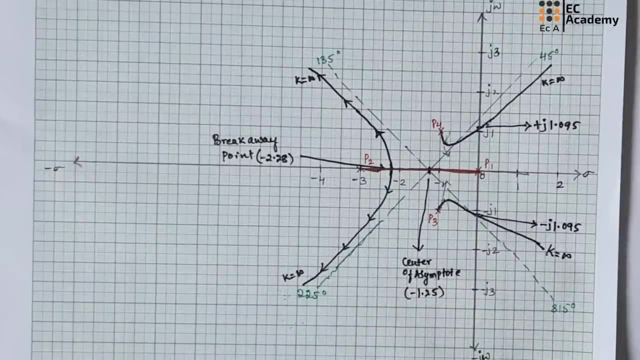 to this line, so it will be up to. K is equal to infinity, so this is the root locus for the given problem. hope you have understood the topic, thank you. 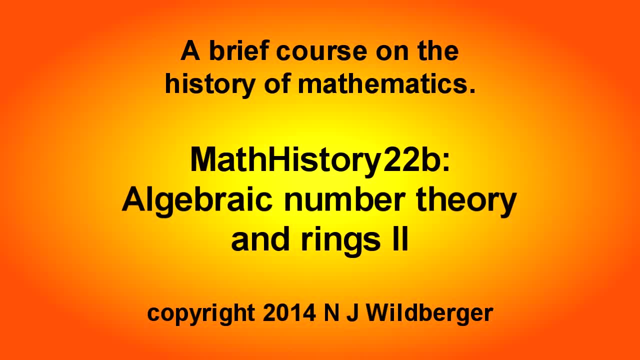 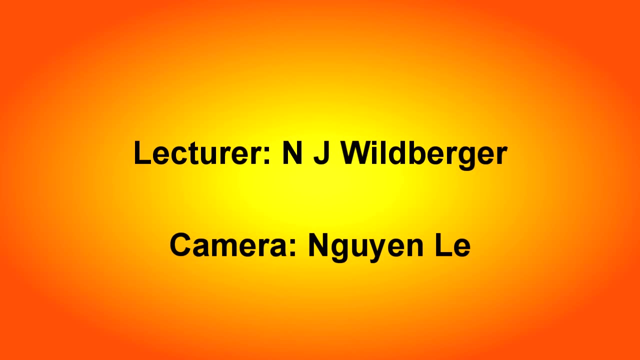 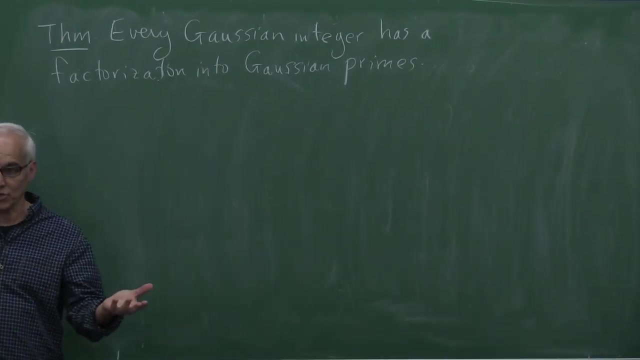 Okay. so a natural question is: we've got these Gaussian integers very simple, just integer combinations of 1 and i and we have this idea of Gaussian primes which is close to being like ordinary primes, but a little bit different. And then the natural question is: does the fundamental 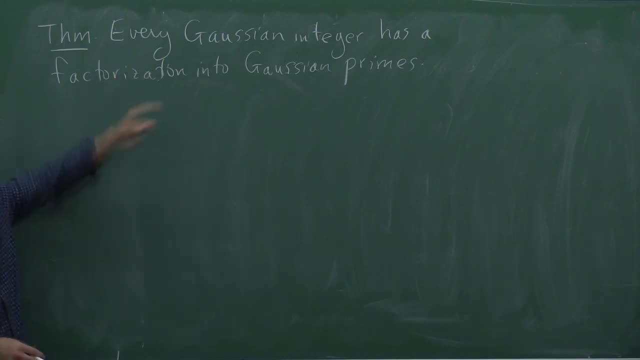 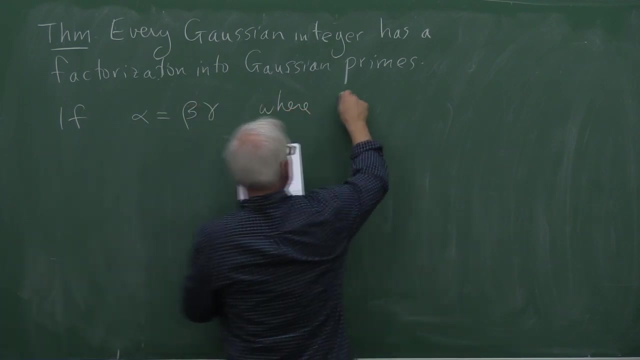 theorem of arithmetic hold. So it's easy to see that every Gaussian integer has a factorization into Gaussian primes. So if alpha is not a prime, then we can write it as a combination of two other Gaussian integers And by the assumptions. this is where q, the quadrants of beta and the 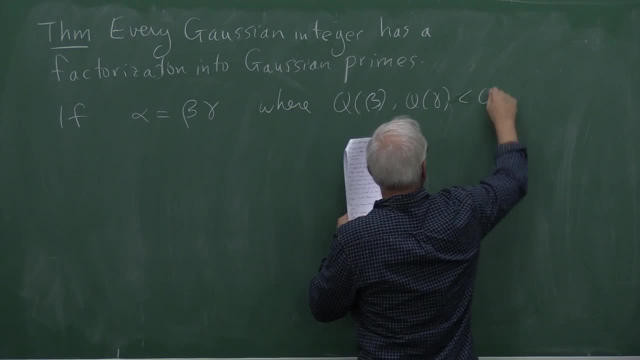 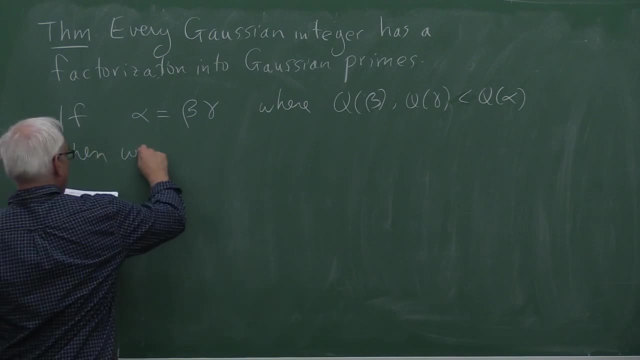 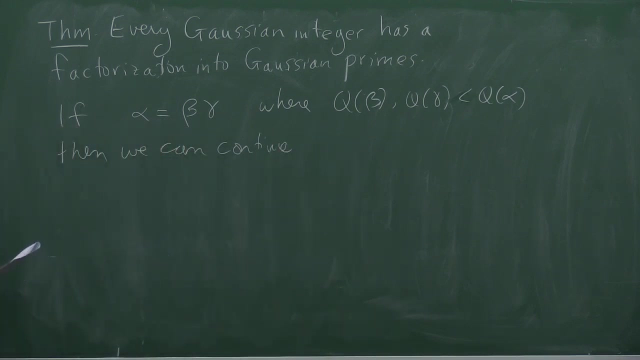 quadrants of gamma equals, is less than the quadrants of alpha. Well, in that case, then we can continue. So we factor it, and if you look at the constituents and if they're not primes, then we write them as products of primes. And we can continue until. 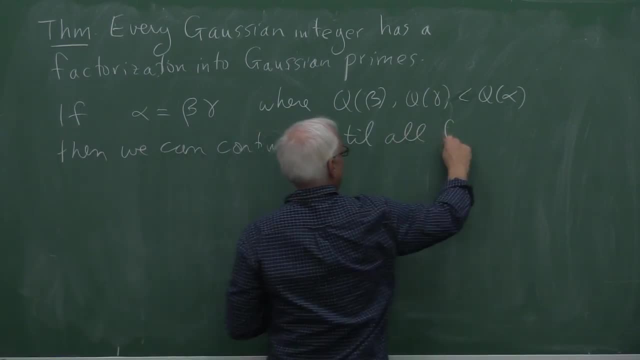 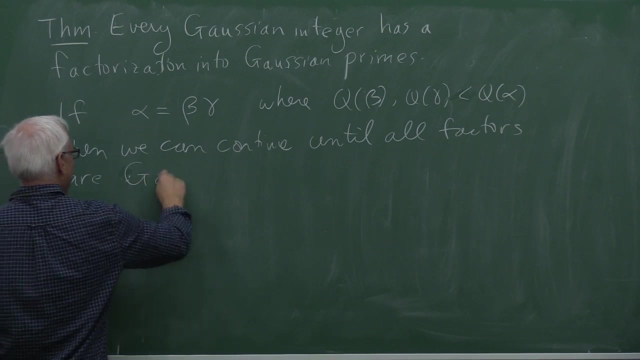 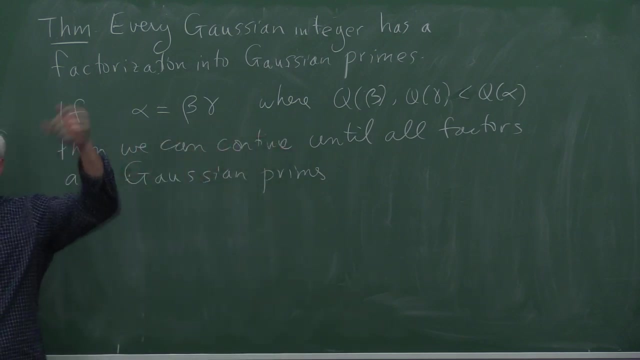 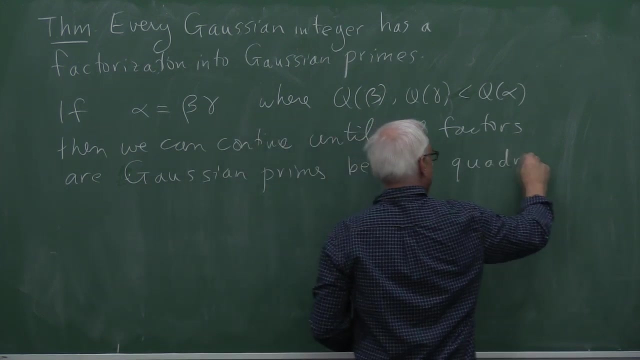 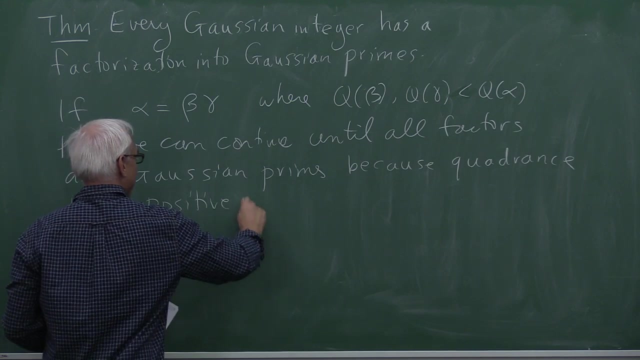 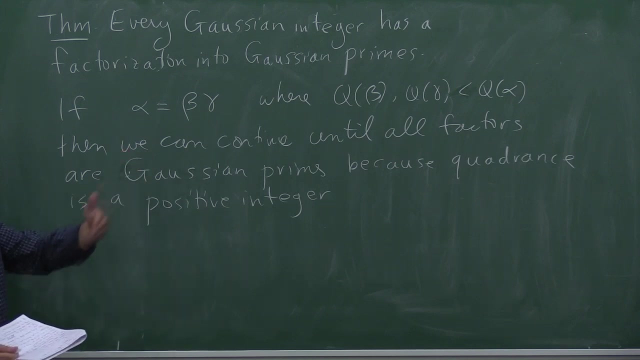 all factors are Gaussian primes, because the quadrants is always a positive integer. Because the quadrants is a positive integer and it must eventually terminate, because there's only a finite number of positive integers less than any given value. So this process must terminate.